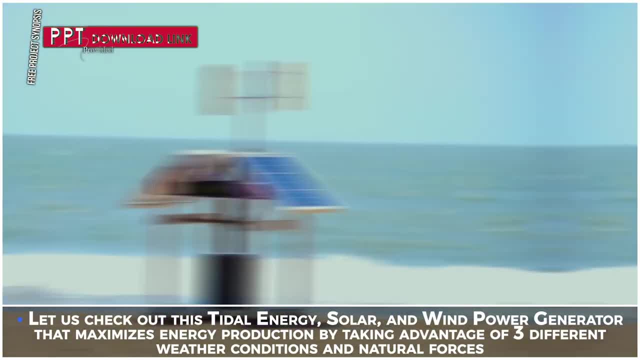 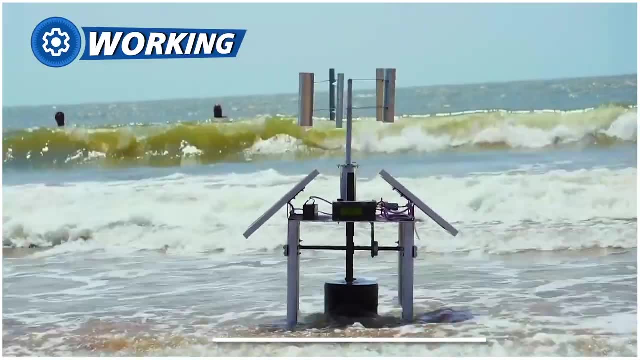 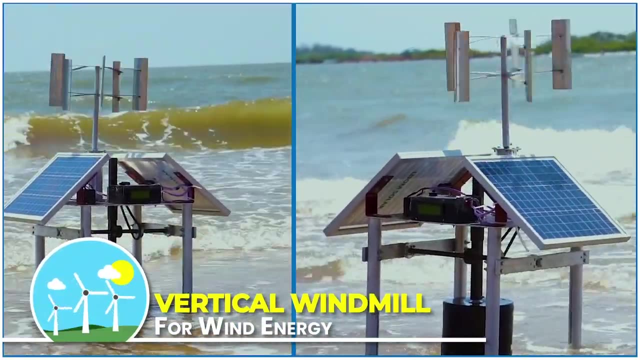 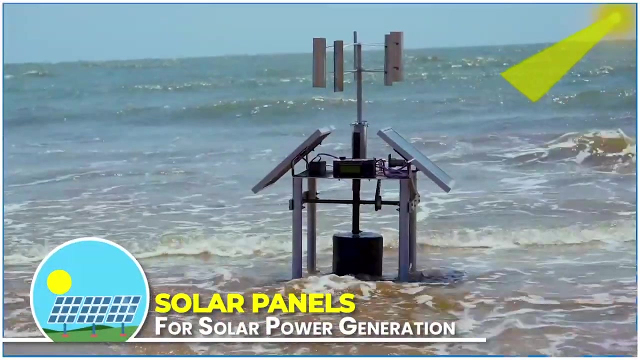 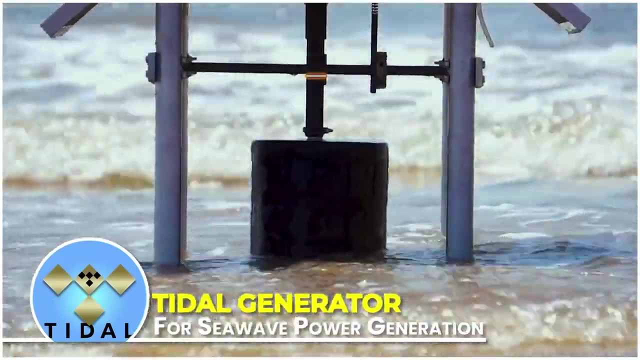 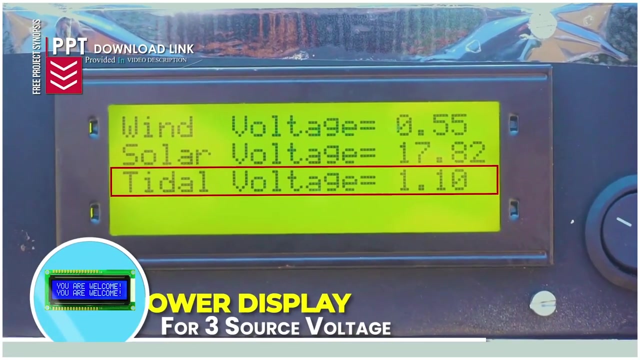 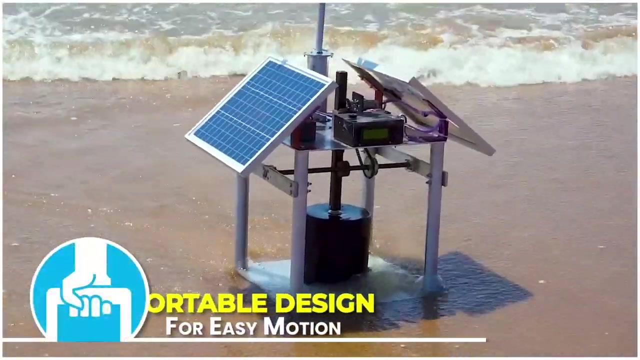 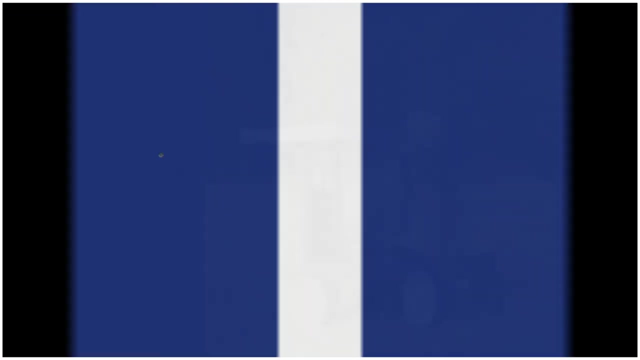 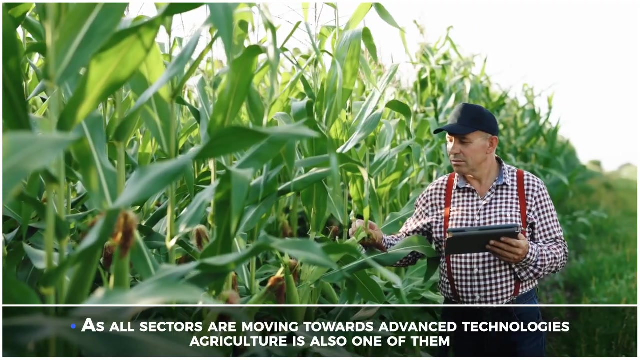 Let us check out this tidal energy, solar and wind power generator that maximizes energy production by taking advantage of three different weather conditions and natural forces. DIY Solar Powered Seed Sprayer Machine. As all sectors are moving towards advanced technologies, agriculture is also one of them. 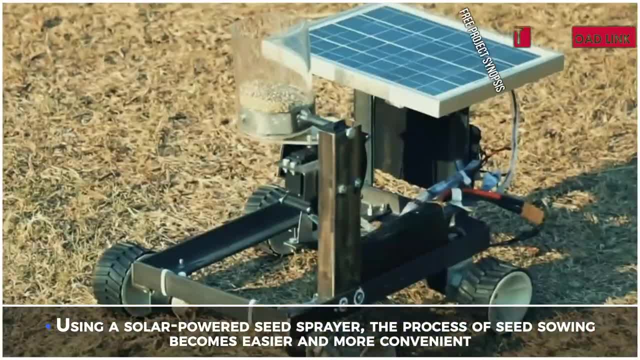 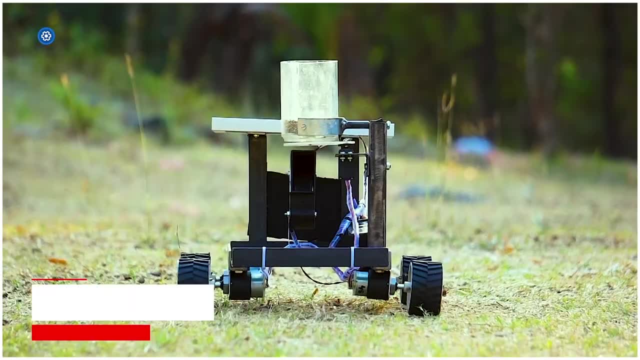 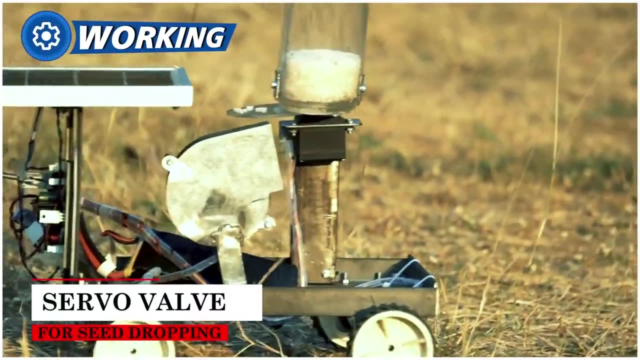 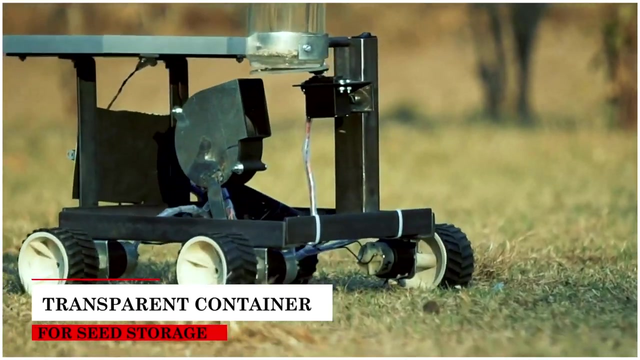 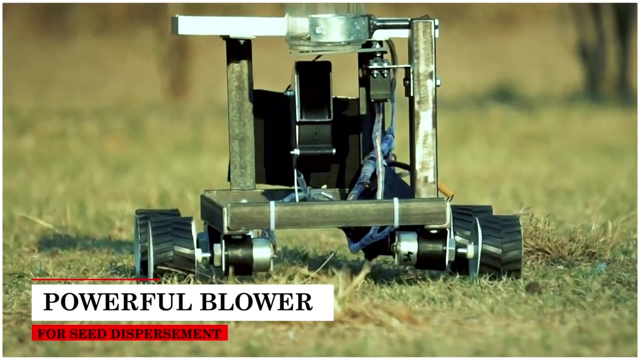 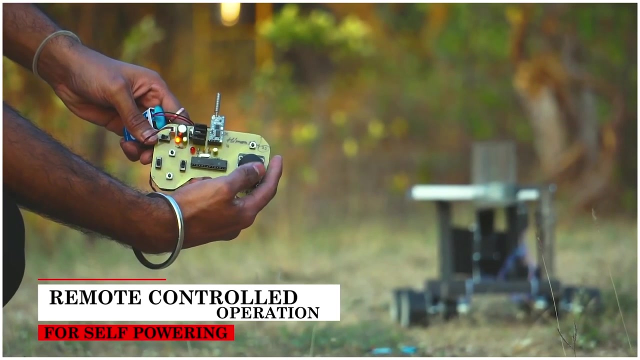 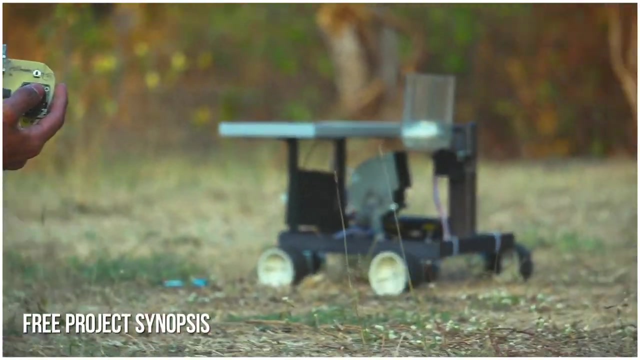 Using a solar powered seed sprayer, the process of seed sowing becomes easier and more convenient. Let's check how this device works without requiring any additional power supply. DIY Solar Powered Seed Sprayer Machine. Dual Power Generation- Solar plus- Windmill Generator. 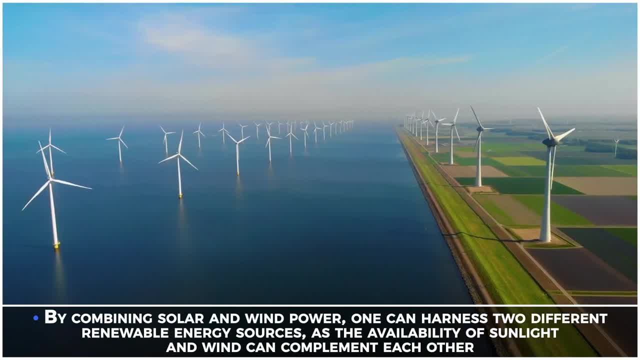 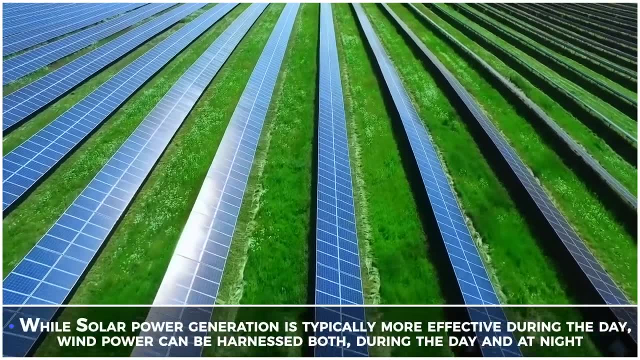 By combining solar and wind power, one can harness two different renewable energy sources, as the availability of sunlight and wind can complement each other. While solar power generation is typically more effective during the day, wind power can be harnessed both during the day and at night. 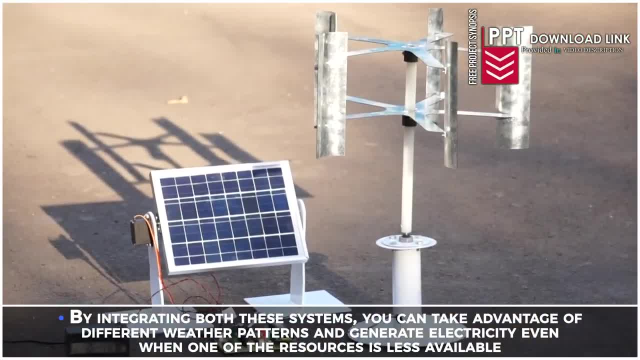 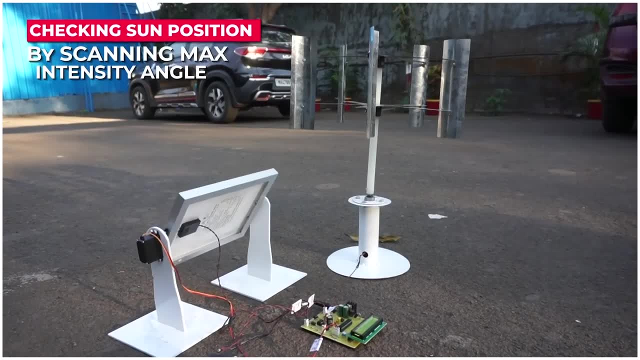 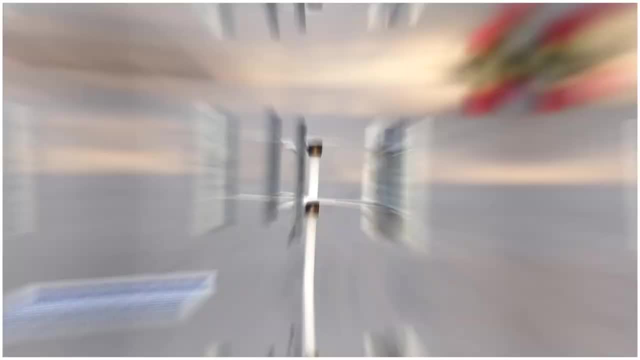 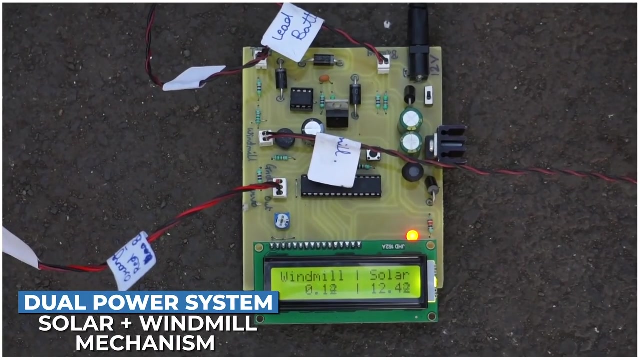 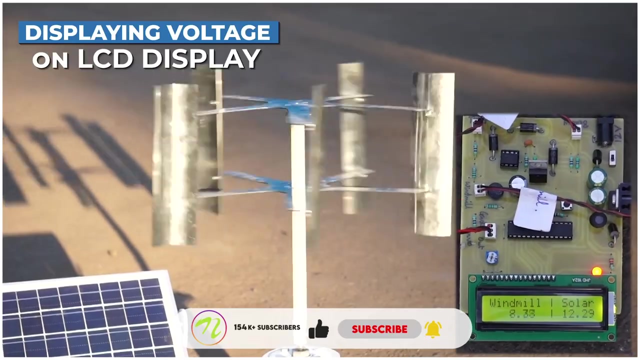 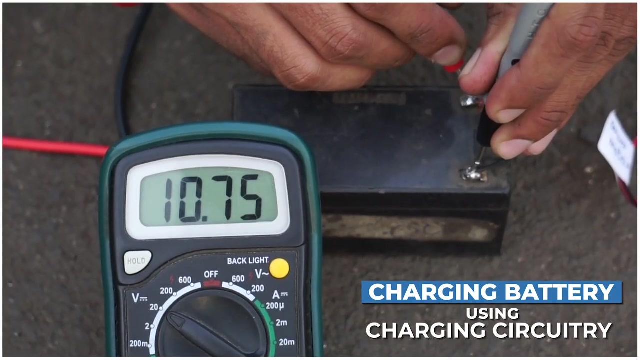 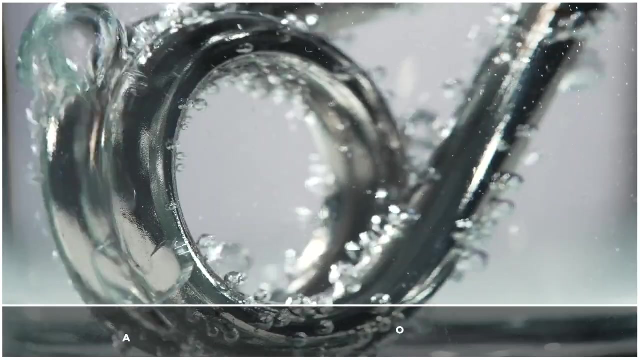 By integrating both these systems, you can take advantage of different weather patterns and generate electricity even when one of the resources is less available. DIY Solar Powered Seed Sprayer Machine. DIY Solar Powered Seed Sprayer Machine. Solar Water Heater for Rooftop. 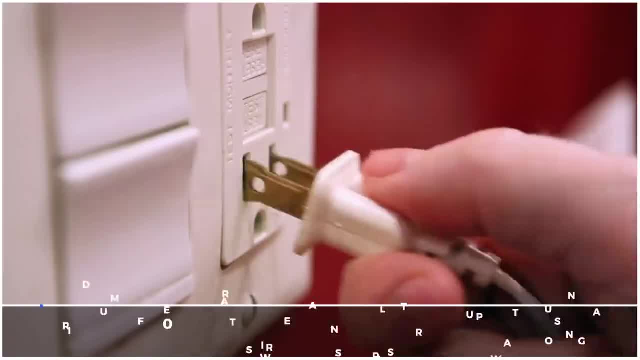 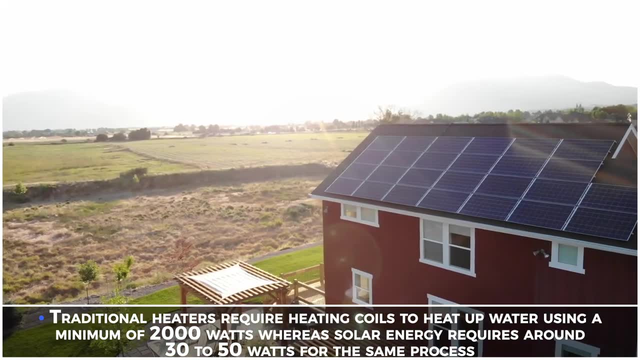 Water heaters consume a large amount of electricity for heating water. Traditional heaters require heating coils to heat up water using a minimum of 2000 watts, whereas solar energy requires a minimum of 600 watts of solar energy. DIY Solar Powered Seed Sprayer Machine. 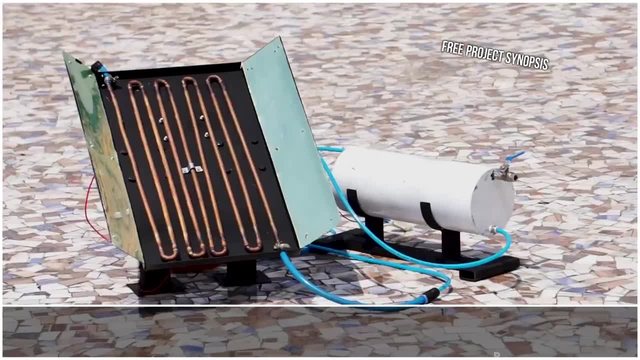 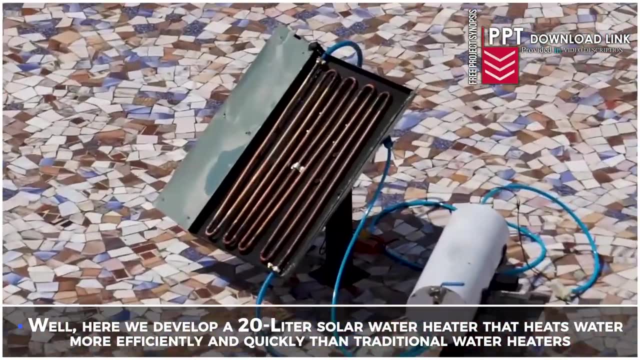 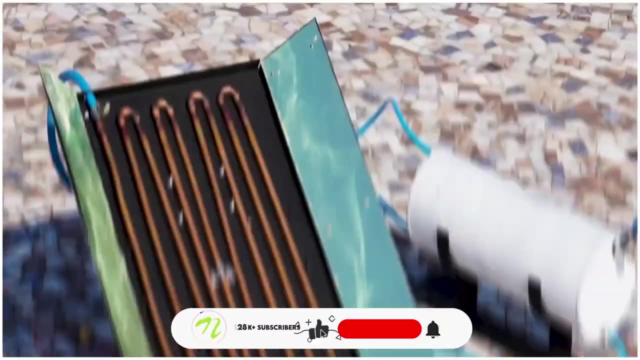 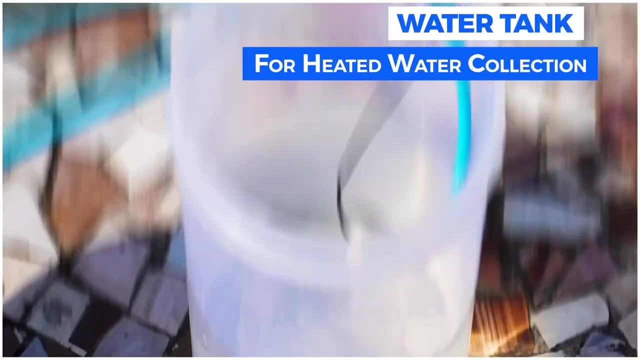 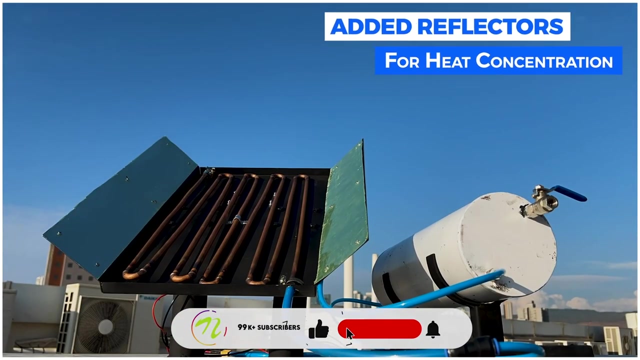 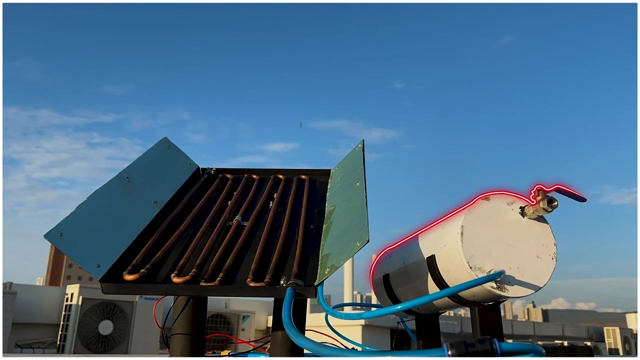 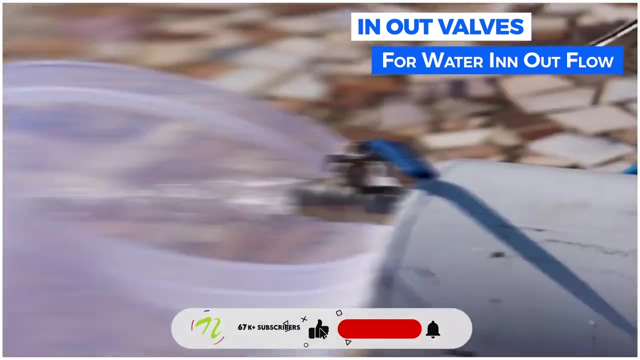 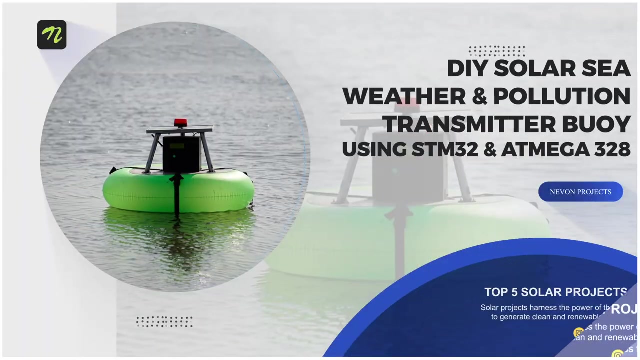 requires around 30-50 watts for the same process. Well, here we develop a 20L Solar Water Heater that heats water more efficiently and quickly than traditional water heaters. DIY Solar Sea Weather and Pollution Transmitter Boy using HTM32 and ATmega328. 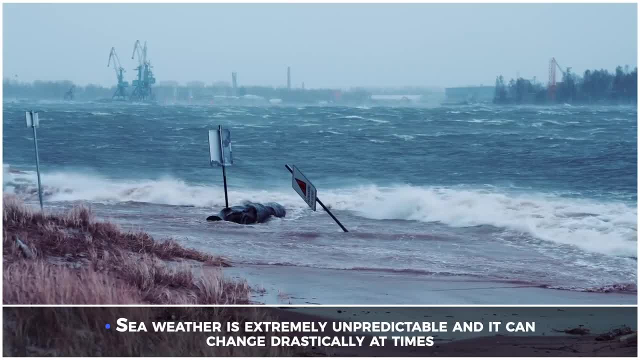 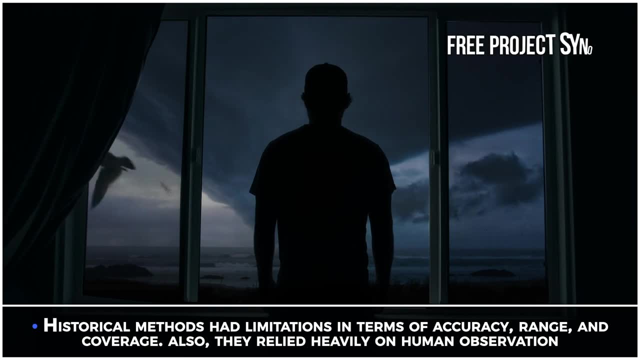 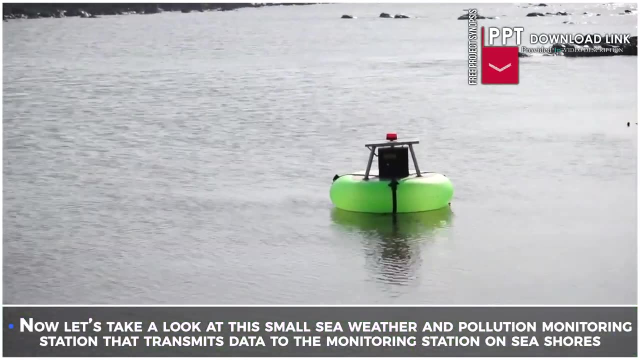 Sea weather is extremely unpredictable and it can change drastically at times. Historical methods had limitations in terms of accuracy, range and coverage. Also, they relied heavily on human observation. Now let's take a look at the Small Sea Weather and Pollution Monitoring Station that transmits data to the monitoring. 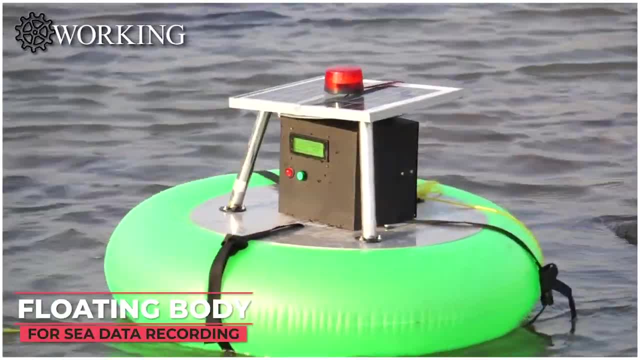 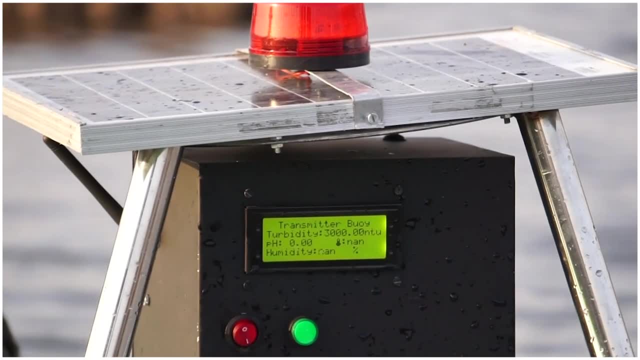 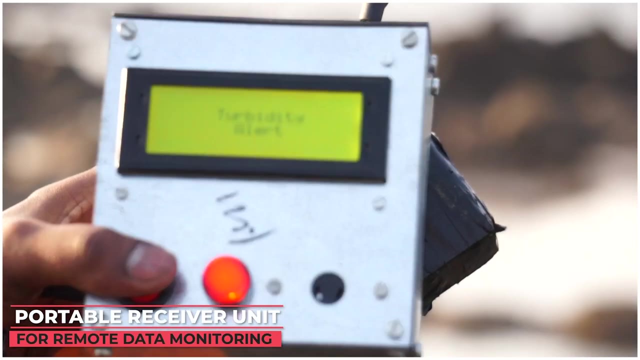 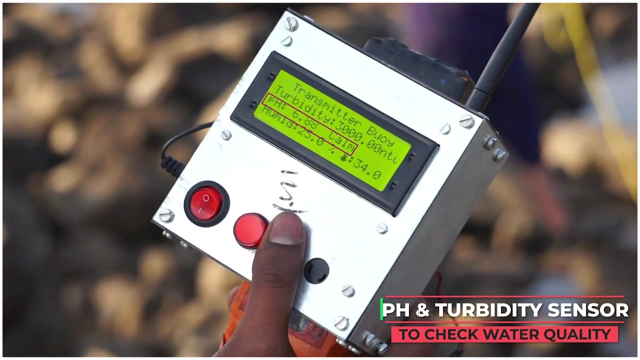 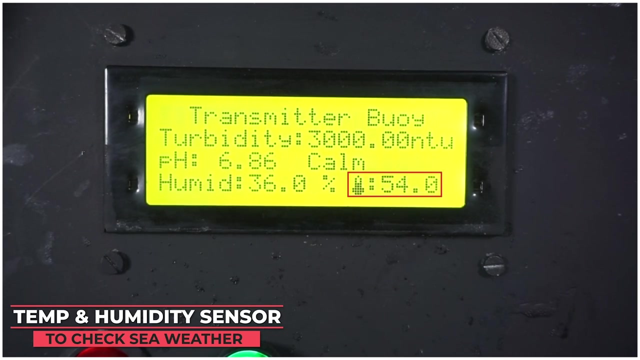 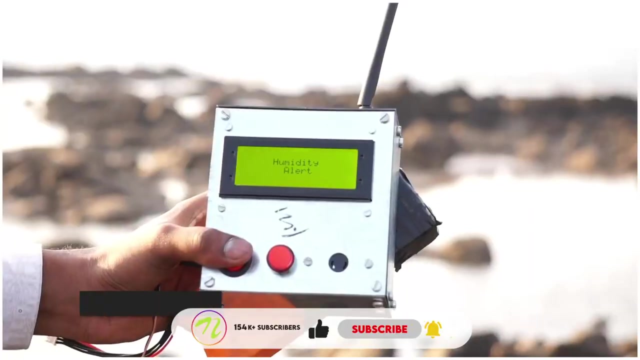 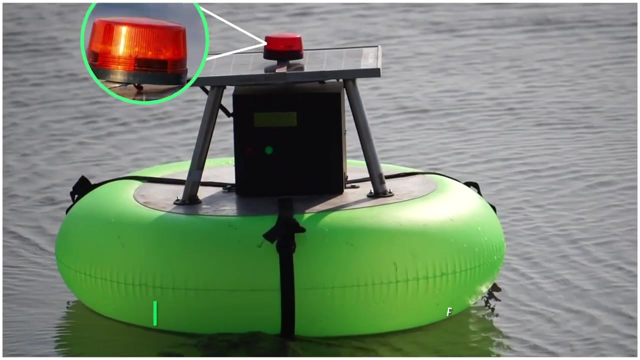 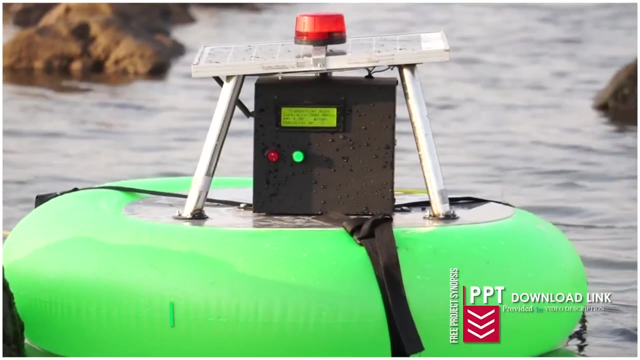 station on seashores. We are testingiga microelectronics to check sieve and be able to mathrunt else an image: вел incisel time condition. Here we can measure travel time. We have a moment that is interesting.